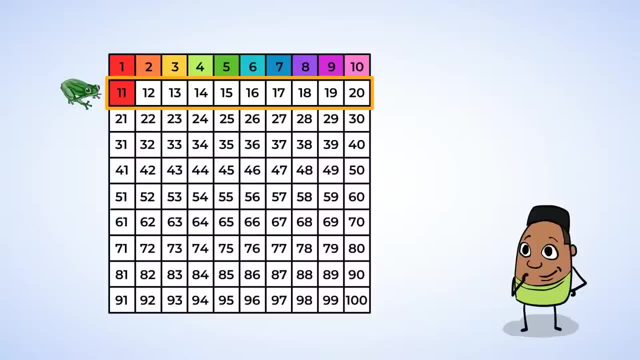 The next row starts with 11.. Then 12,, 13,, 14.. 15,, 16,, 17,, 18,, 19,, 20.. Okay, on to the next row. Ready froggy Jump. 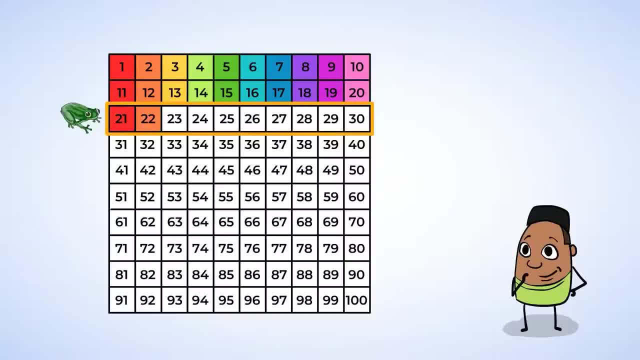 And here we have 21,, 22,, 23,, 24,, 25,, 26,, 27,, 28,, 29,, 30.. One more row, And then we're going to take a quick break. Ready froggy. 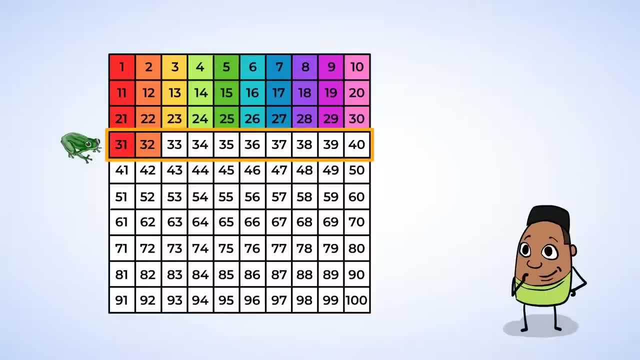 Jump: 31,, 32,, 33,, 34,, 35,, 36,, 37,, 38,, 39, 40.. Whoa, Okay, now we've counted so many numbers already. I think it's good to stop for a minute and take a look at them. 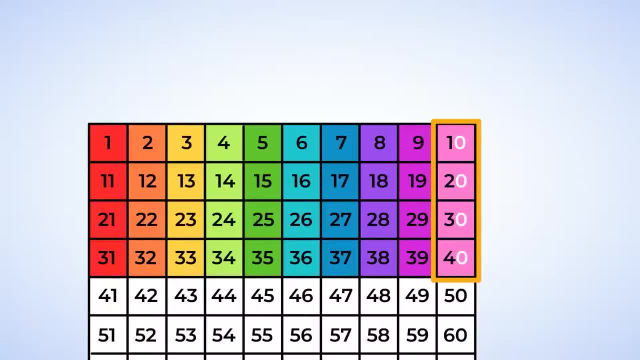 But look at the pink numbers. They all have a zero in them. What were their names? again, 10.. Oh yeah, that's right. 10, 20,, 30,, 40.. Let's take a look at the rest of the numbers in this pink column before going on. 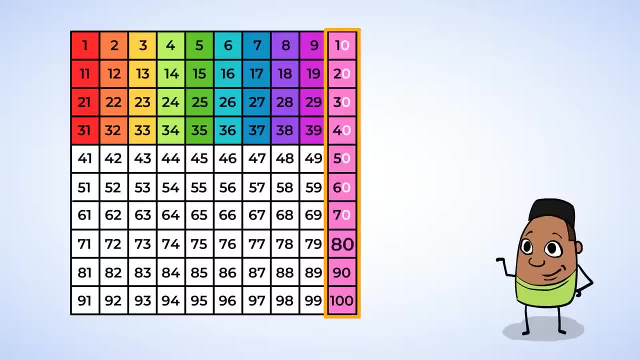 50,, 60,, 70,, 80,, 90, 100.. Okay, these numbers all have zeros at the end, And knowing their names will help with the rest of our counting. Uh, but where did we leave off before? 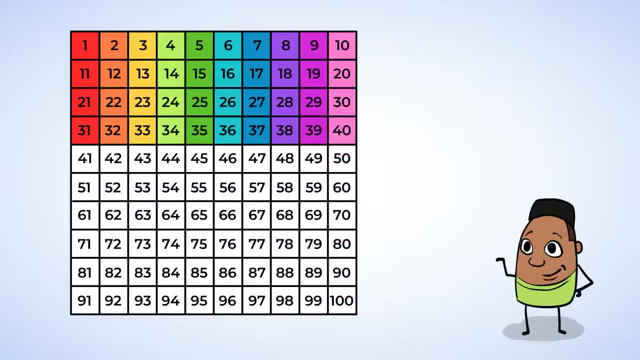 Oh yeah, that's right. 38,, 39,, 40.. Right Now, what comes next? Well, look at the red numbers In this red column. they all have a 1 at the end: 1,, 11,, 21,, 31.. 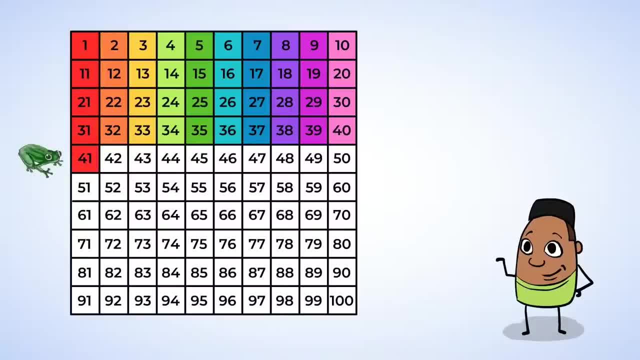 So after 40 comes 41.. And next the orange numbers all have a 2 at the end: 2,, 12,, 22,, 32.. So after 41 is 42.. Okay, let's just finish this row now. 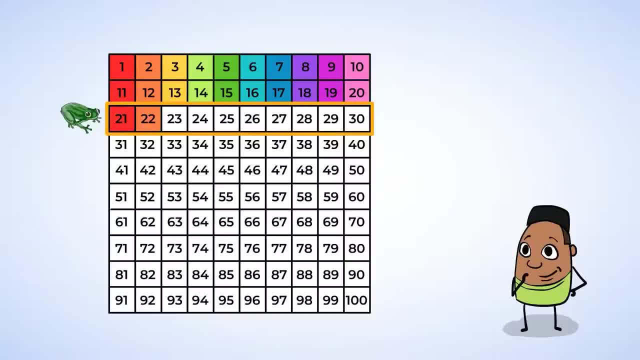 And here we have 21,, 22,, 23,, 24,, 25,, 26,, 27,, 28,, 29,, 30.. One more row, And then we're going to take a quick break. Ready froggy. 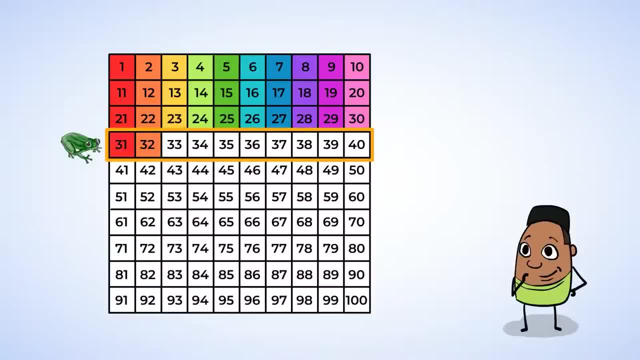 Jump: 31,, 32,, 33,, 34,, 35,, 36,, 37,, 38,, 39, 40.. Whoa, Okay, now we've counted so many numbers already. I think it's good to stop for a minute and take a look at them. 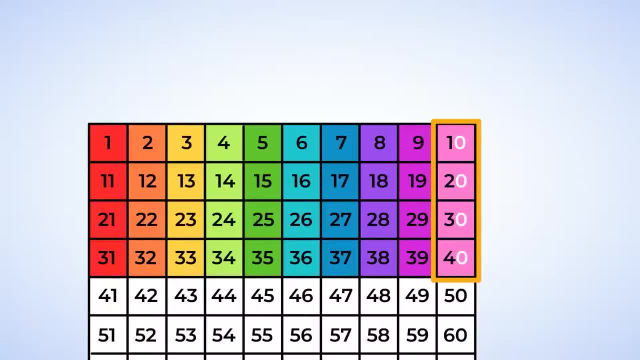 But look at the pink numbers. They all have a zero in them. What were their names? again, 10.. Oh yeah, that's right. 10, 20,, 30,, 40.. Let's take a look at the rest of the numbers in this pink column before going on. 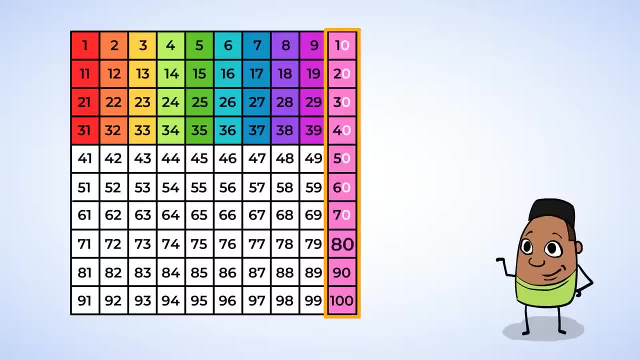 50,, 60,, 70,, 80,, 90, 100.. Okay, these numbers all have zeros at the end, And knowing their names will help with the rest of our counting. Uh, but where did we leave off before? 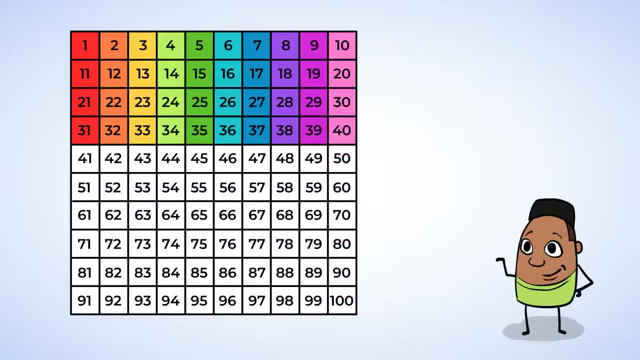 Oh yeah, that's right. 38,, 39,, 40.. Right Now, what comes next? Well, look at the red numbers In this red column. they all have a 1 at the end: 1,, 11,, 21,, 31.. 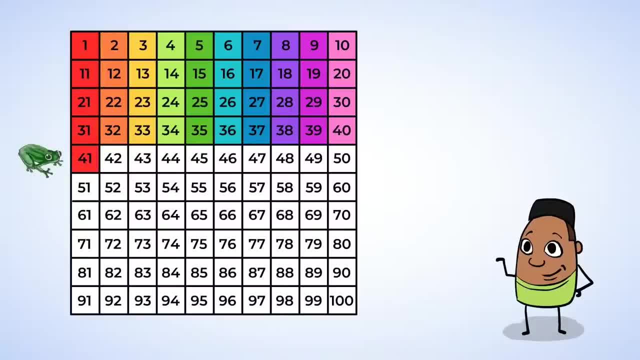 So after 40 comes 41.. And next the orange numbers all have a 2 at the end: 2,, 12,, 22,, 32.. So after 41 is 42.. Okay, let's just finish this row now. 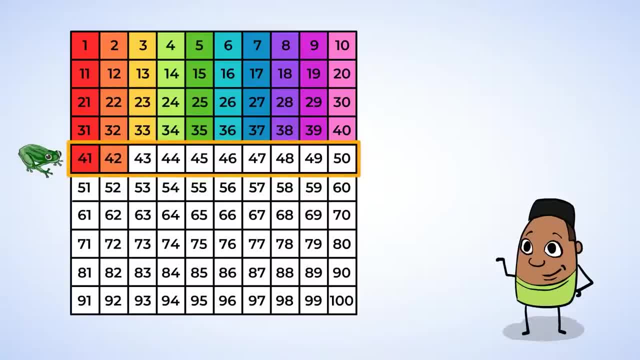 We already have 41.. 41 and 42., Then next is 43,, 44,, 45. And after 45 is 46,, 47,, 48,, 49,, 50. Froggy jump, Wow, we're already counting so high. 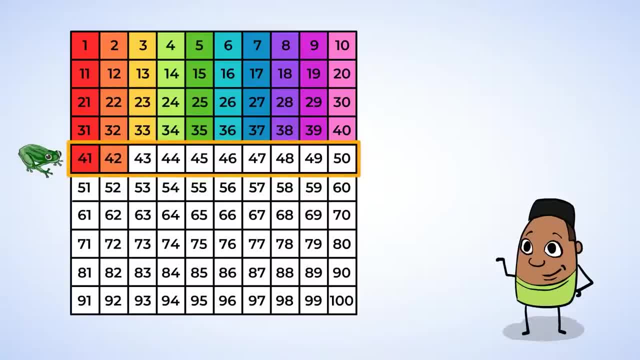 We already have 41.. 41 and 42., Then next is 43,, 44,, 45. And after 45 is 46,, 47,, 48,, 49,, 50. Froggy jump, Wow, we're already counting so high. 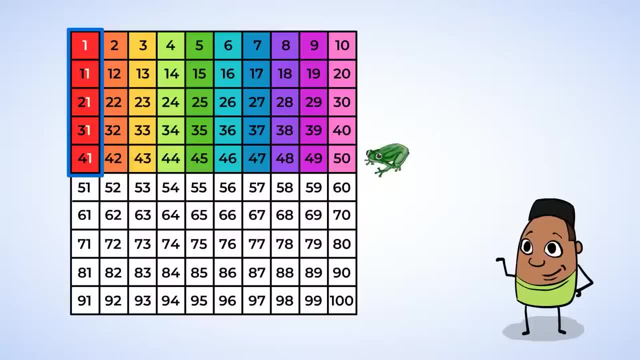 Look at the red column. Remember each number has a 1 at the end. So what comes after 50?? Well, next comes 51. Then 52., Then 53. And if you forget, just look at the end of the last number you counted. 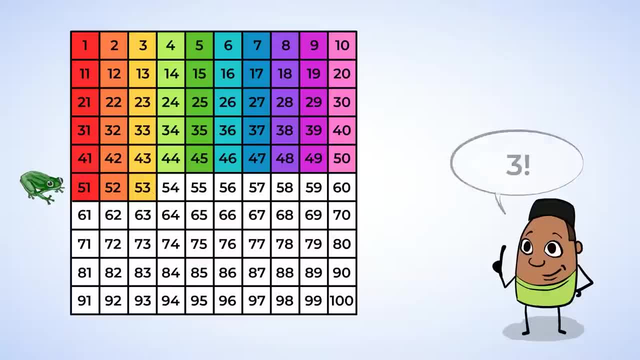 At the end of 53 is a 3. So what comes after 3?? 4. So after 53 is 54. That's right. Then 55. Then 56. And what comes after 56?? Well, what comes after 6?? 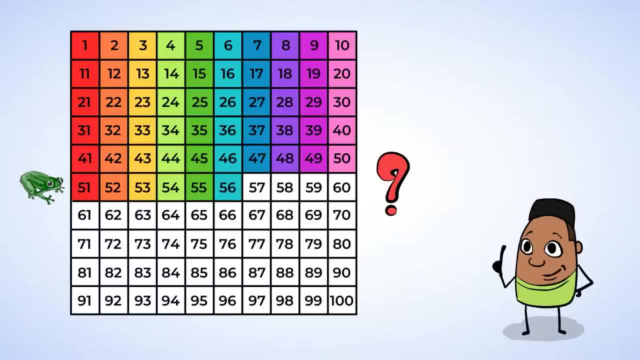 7. So after 56 is 57. Then 58. Then 59. And 60. After 59 is 60. Because after 5 is 6. Then since a 0 is at the end of 60., 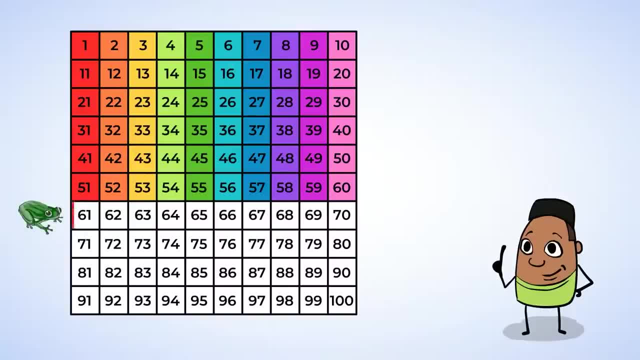 Uh, Froggy, would you please? We start all over again with 61., 62., 63., 64. And what comes next? Well, look at all the dark green numbers. What's at the end of all those numbers? 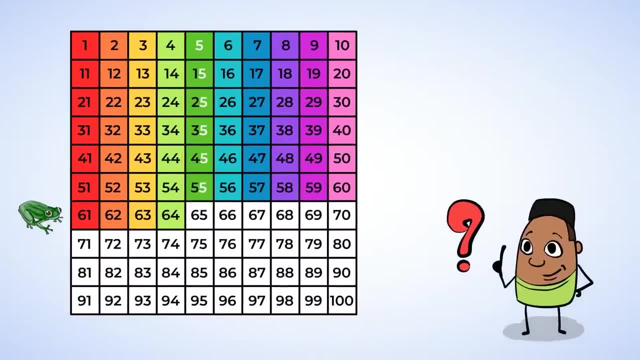 5. That's right. So after 64 is 65. Then 66., 67., 68., 69., 70. And you know what comes next: 71. And after 71 is 72. And you know what comes next. 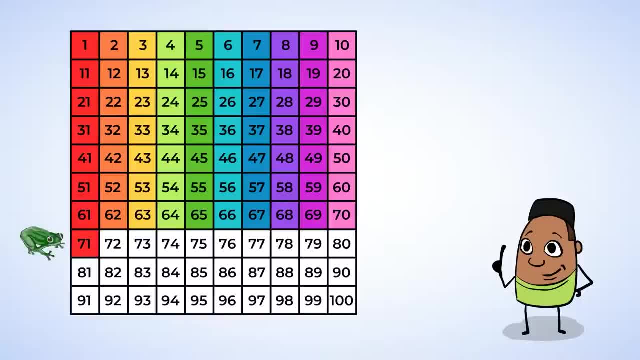 71. And after 71 is 72. And you know what comes next: 71. And after 71 is 72.. And you know what comes next: 71., 72., 73., 74., 75.. 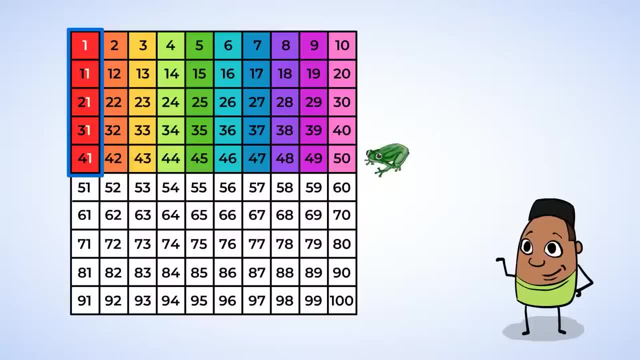 Look at the red column. Remember each number has a 1 at the end. So what comes after 50?? Well, next comes 51. Then 52., Then 53. And if you forget, just look at the end of the last number you counted. 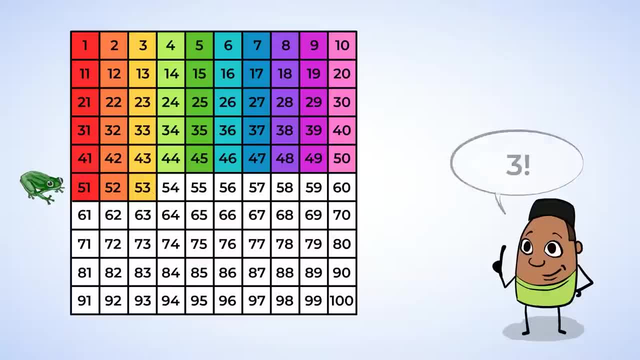 At the end of 53 is a 3. So what comes after 3?? 4. So after 53 is 54. That's right. Then 55. Then 56. And what comes after 56?? Well, what comes after 6?? 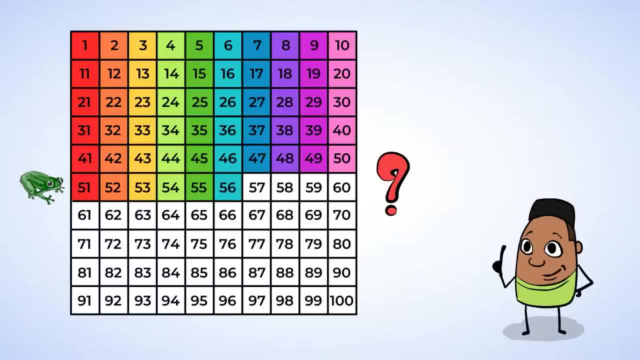 7. So after 56 is 57. Then 58. Then 59. And 60. After 59 is 60. Because after 5 is 6. Then since a 0 is at the end of 60., 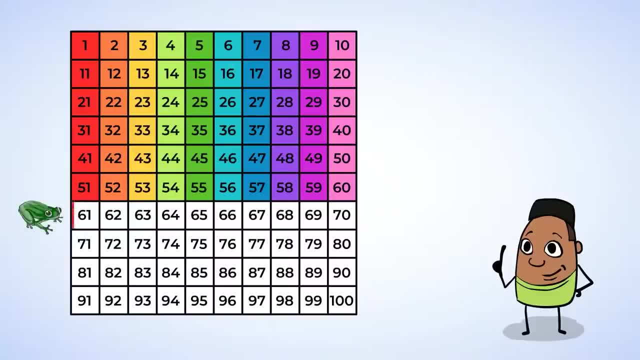 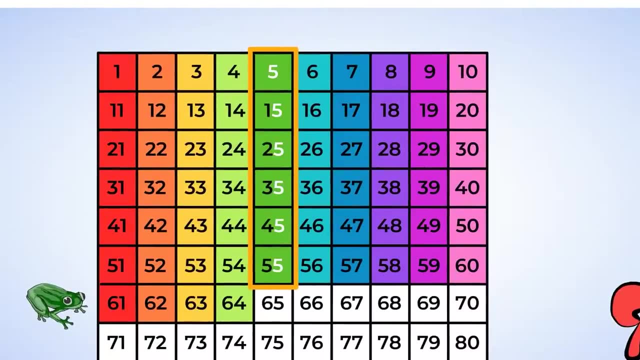 Uh, Froggy, would you please? We start all over again with 61., 62., 63., 64. And what comes next? Well, look at all the dark green numbers. What's at the end of all those numbers? 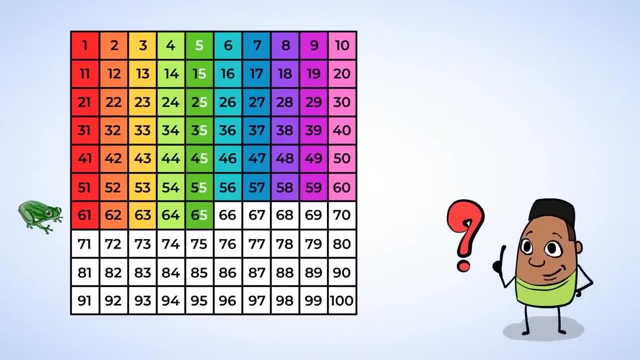 5. That's right. So after 64 is 65. Then 66., 67., 68., 69., 70. And you know what comes next: 71. And after 71 is 72. And you know what comes next. 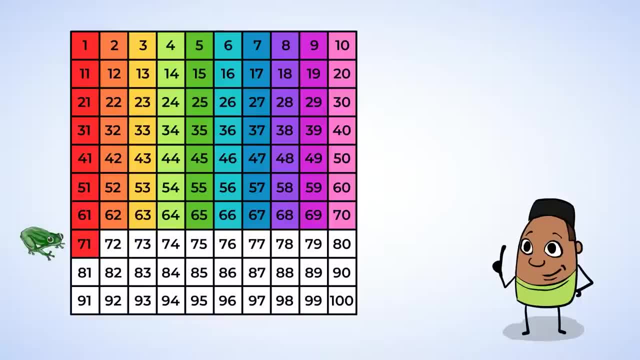 71. And after 71 is 72. And you know what comes next: 71. And after 71 is 72.. And you know what comes next: 71., 72., 73., 74., 75.. 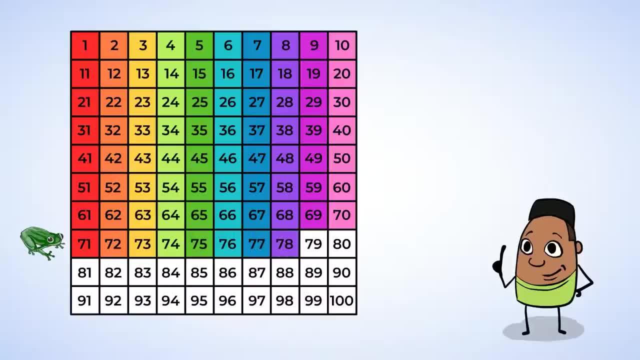 76., 77., 78., 79. 80.. Just like before, all of the red numbers have a 1 at the end. So after 80 we start with, come on Froggy 81. Then 82.. 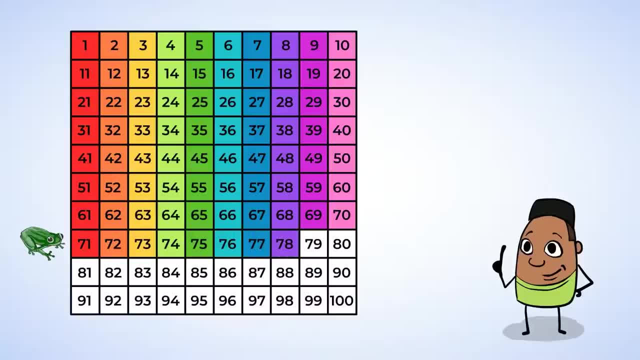 76., 77., 78., 79., 80.. Just like before, all of the red numbers have a 1 at the end. So after 80, we start with, come on Froggy 81. Then 82.. 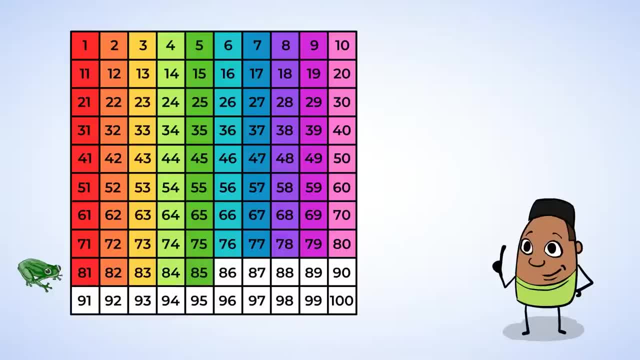 Then 83., 84., 85. And after 85 comes. well, let's look at the light blue numbers. They all end in 6.. So after 85 is 86. And then 87., 88., 89.. 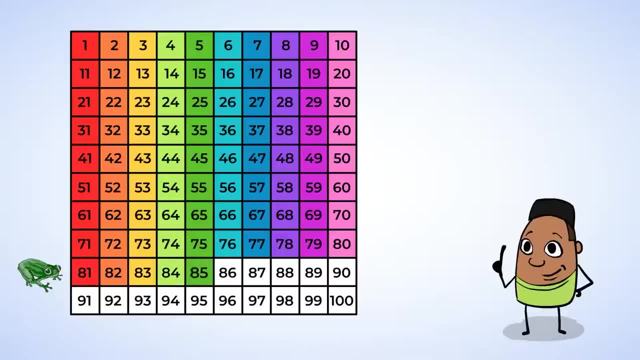 Then 83., 84., 85. And after 85 comes. well, let's look at the light blue numbers. They all end in 6.. So after 85 is 86. And then 87., 88., 89.. 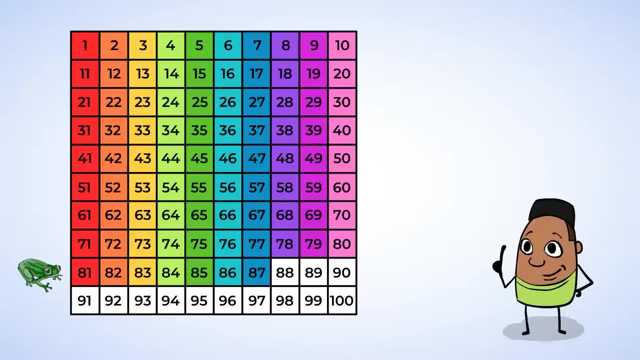 90.. Wow, We only have one more row to go. You've counted all the way up to 90 so far. Come on, Froggy, let's jump on down to the final row. What comes after 90?? You got it. 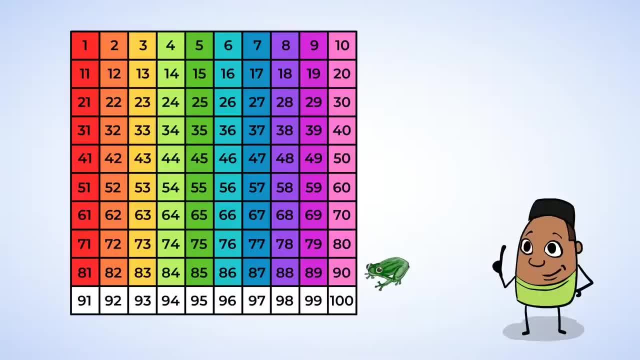 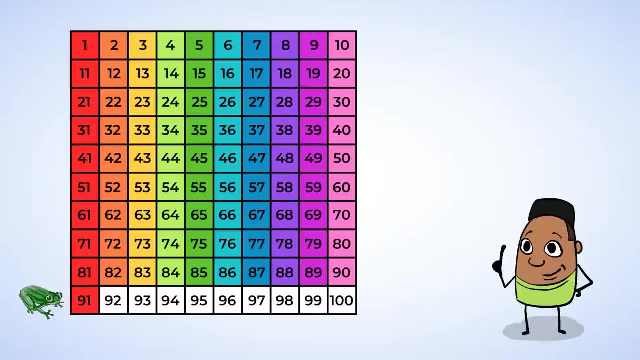 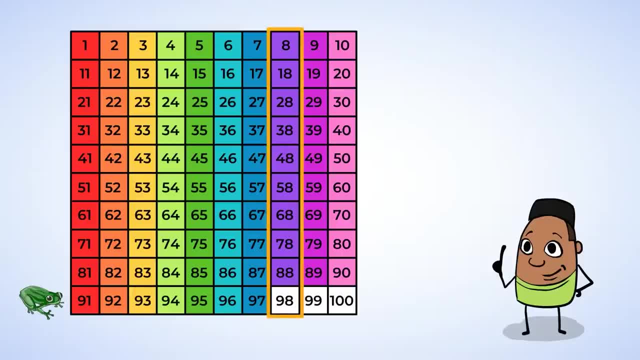 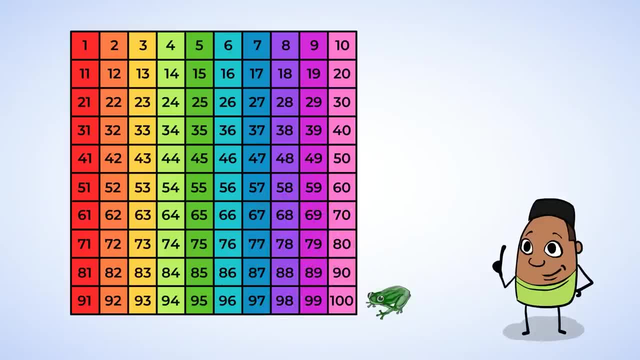 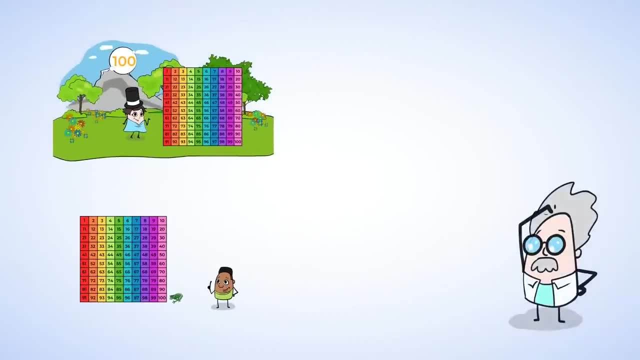 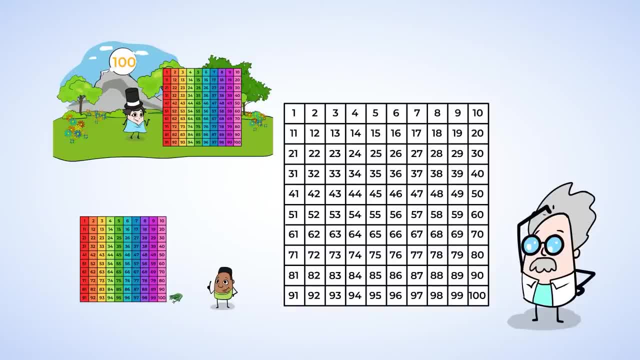 on your own using the hundreds chart And as you're counting, try coloring your own chart just like this one, And you can always come back to this video if you want to count to 100 again. Until then, see you in the next video, my mighty friend.